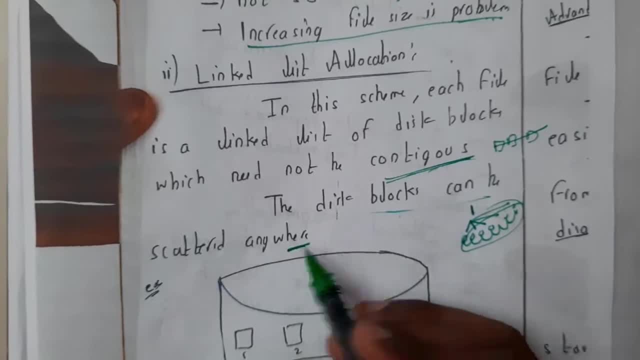 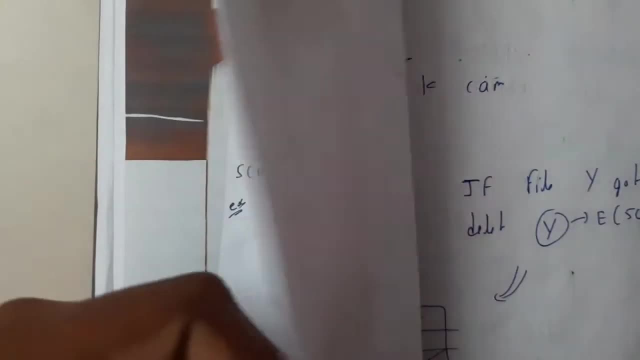 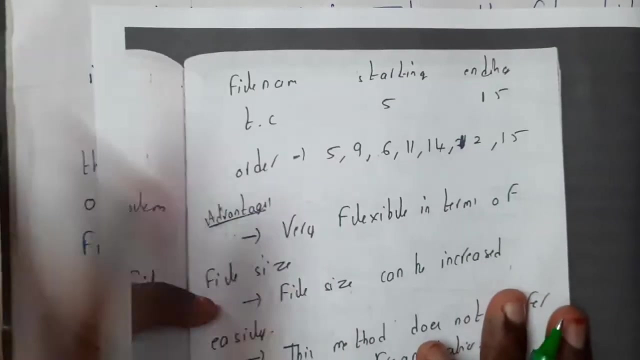 can be scattered anywhere, So the disk blocks can be scattered. That's what the next point is: The disk blocks can be scattered anywhere. So here we will be taking the small table, guys, which consists of starting, ending and the order in which the links. That is, nothing but the linked. 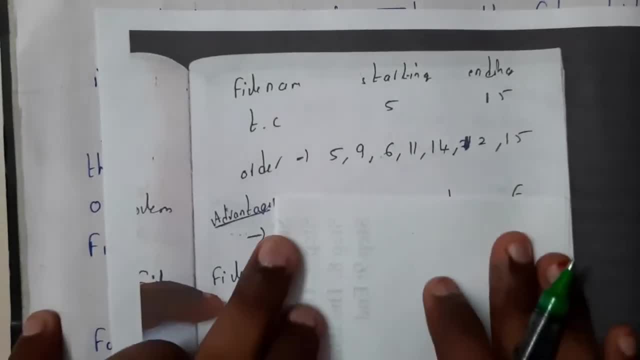 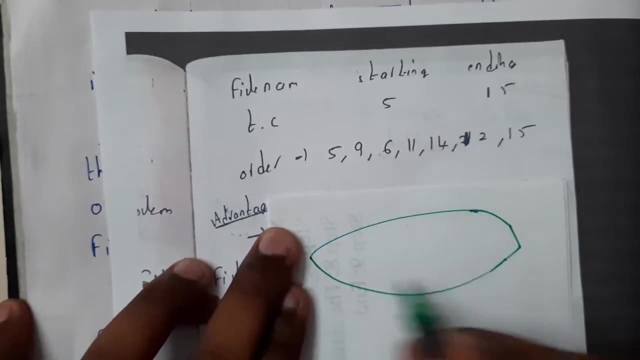 list order. Okay, so if you want me to draw, I will be just drawing it here again, Like previously we have drawn Okay. so basically let me draw it first. So till 16, only right. So let me take neatly at least. now Let me try. 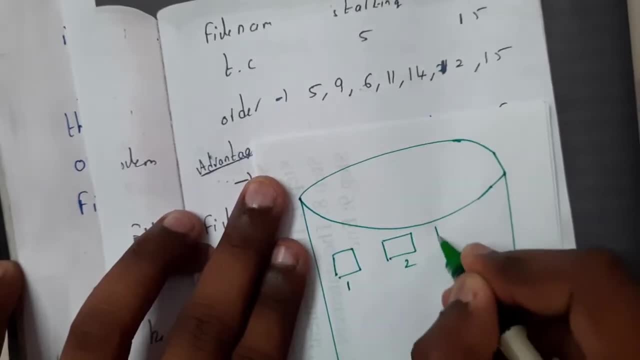 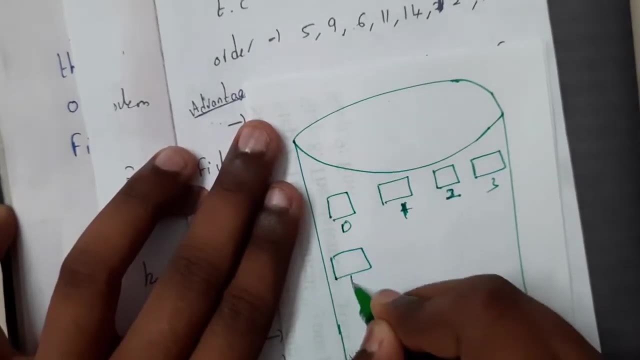 One. I will be writing it outside, guys for that Now for now, Three. Okay, let me start it from zero. only That's better. One, two, three, four, five, six, seven, eight, nine, ten. 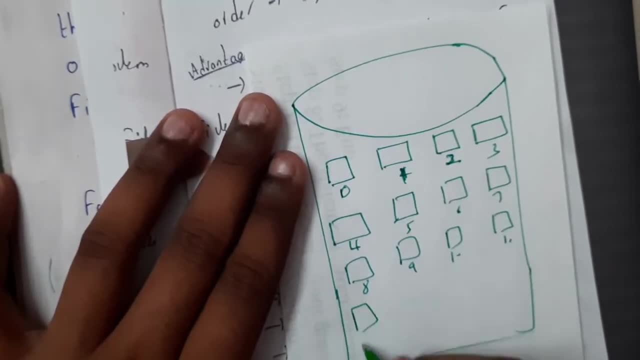 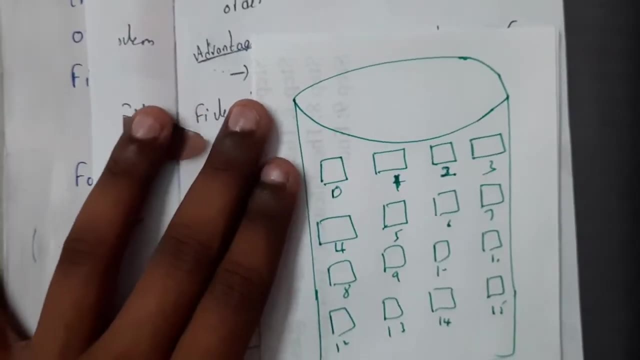 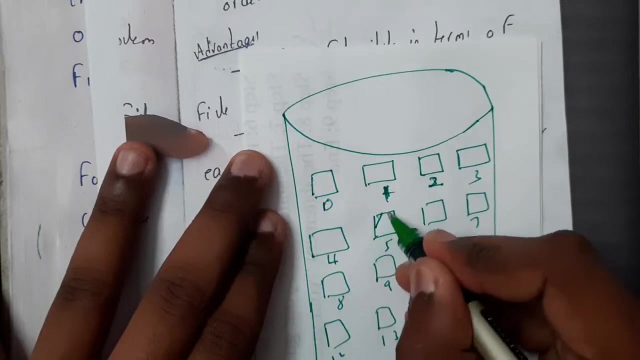 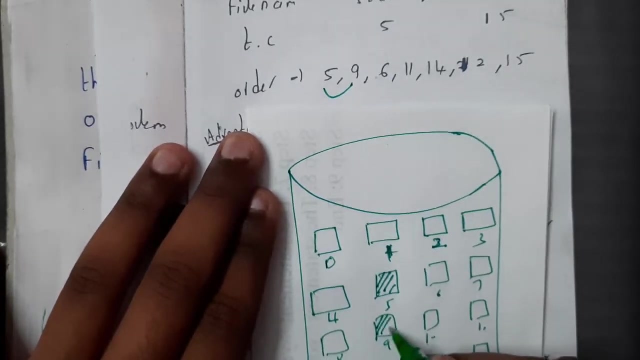 Eleven, Twelve, Thirteen, Fourteen, Fifteen. I think you have exactly filtered them, Yeah, 15.. Fine, Okay. So he told that the starting is five and ending is nine. So starting is five. Okay, from five we went to nine. Okay, where is nine? Here it is nine. So now you will be. 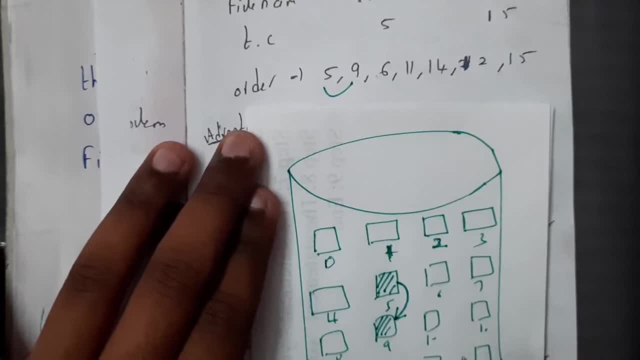 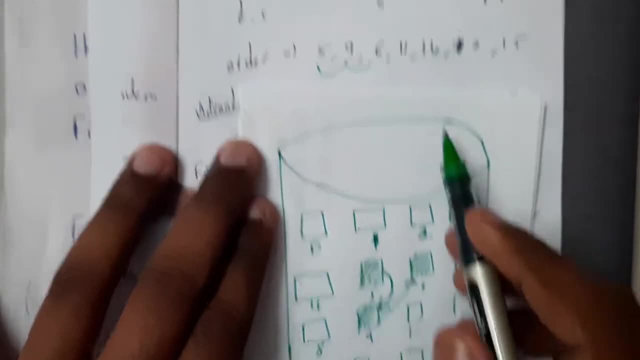 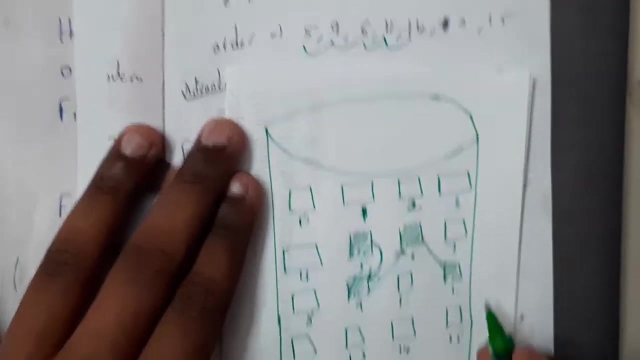 establishing a link in between them. Okay, we established them. After that 9, we need to go to 6. so 6 is right here. move, highlight it. after that, from 6, we will be going to 11. so 10, 11, it's here. from 11, you'll be going to 14. here, guys. 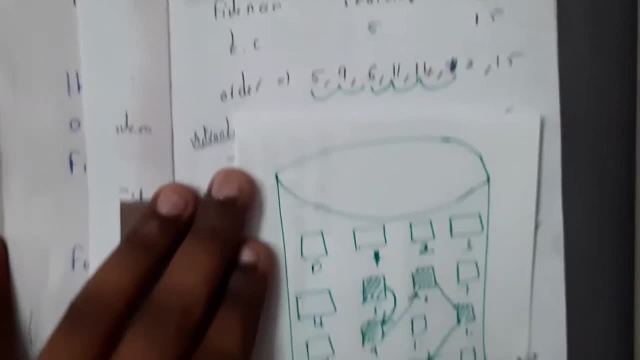 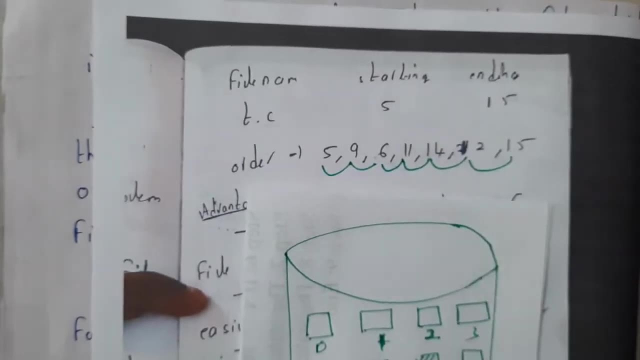 don't forget to keep arrows, guys, because at the end you'll be confused. to keep arrows. if you forget to keep arrows, you'll be confused at the end. to which direction should I keep? okay, after 2 will go back to 15, get to the end, so we. 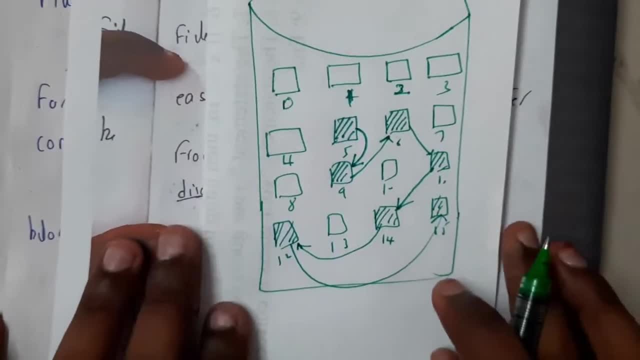 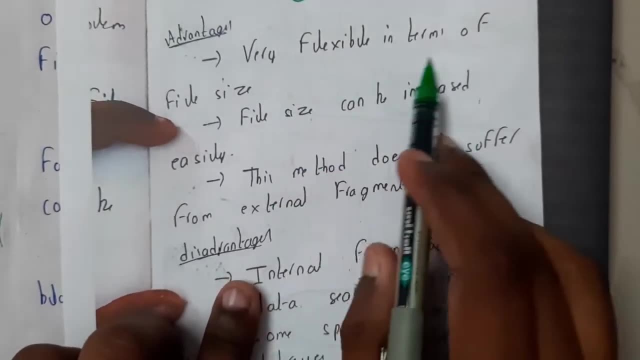 started at 5 and we ended at 15. so this is our linked list allocation of the given file. so I hope everyone got a small idea on this. so now let us go through advantages. so very flexible in terms of file size, because, if I want to, 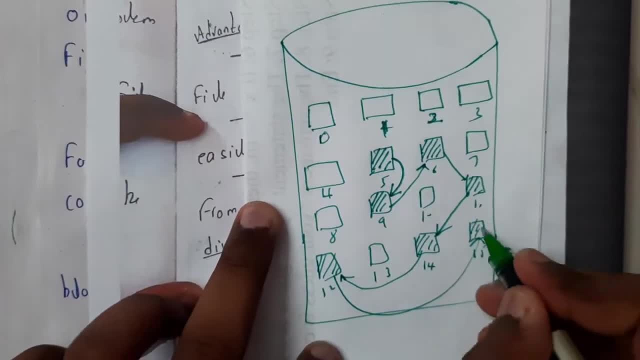 increase the file size, so I'll be just adding: from 15 I'll be moving to 7, from 7 I'll be moving to 3, from 3 to 2, 3, 2 to 1, 2 to 0, 1 to 0 and I'll be changing. 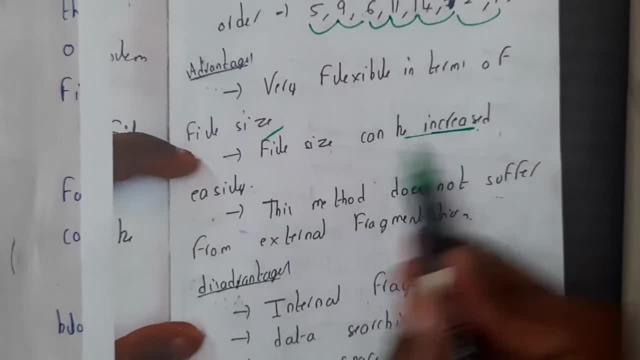 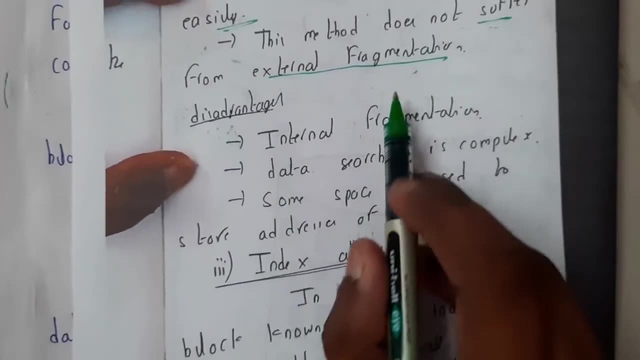 this end to 0. that's it, so I can expand my file, right. so that's the main advantage here, and the method does not suffer from external fragmentation. so there is no chance of external fragmentation, guys. fine, and the disadvantages we will be facing from internal fragmentation and 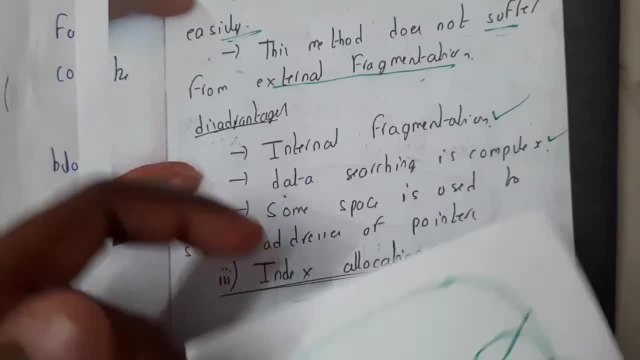 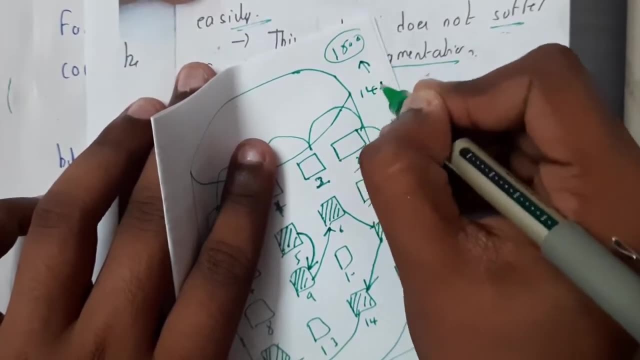 data searching is a bit complex. so let us assume your linked list is consisting of 1500 keys or values, so you want to search a last 148th value or 1488th value. so how much time will it take? as because the searching time will take. 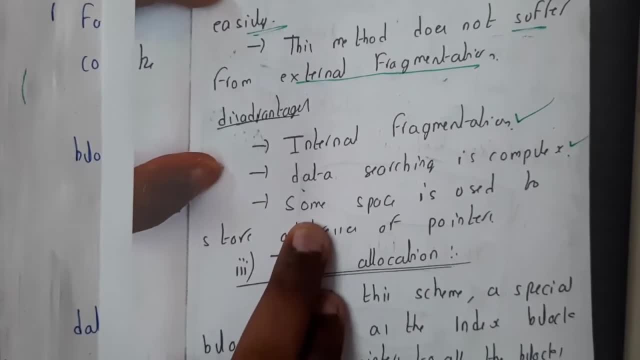 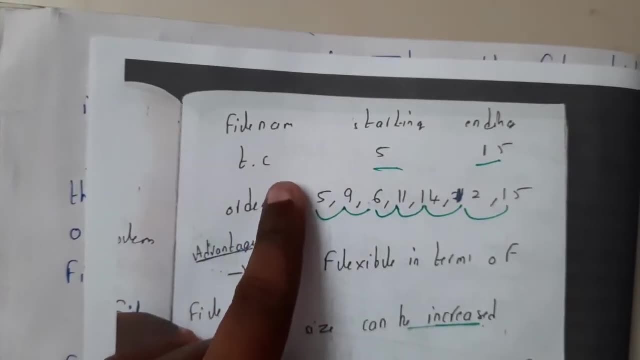 really long, so that's the main reason. some space is used for storing the data of the file, so that's the main reason. some space is used for storing the data of the pointers, so you need to store this right, so some space is wasted. fine, so I hope. 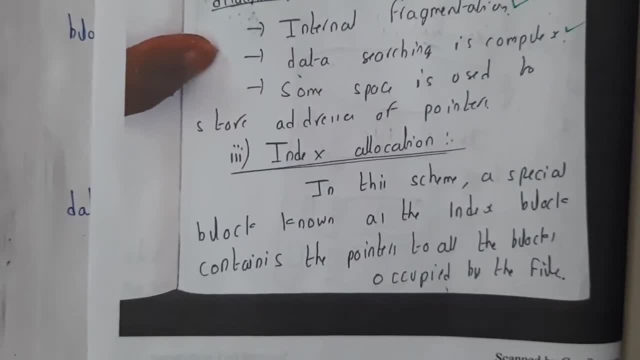 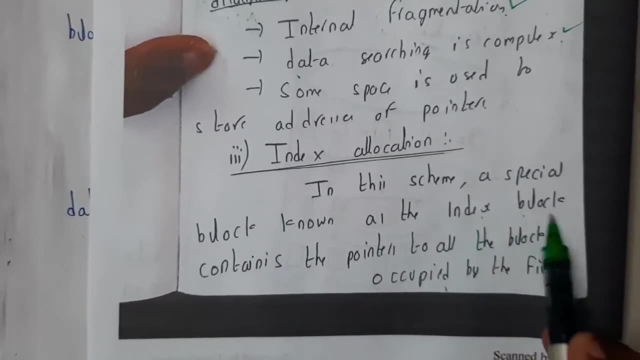 everyone got a small idea on this, so now let us continue with indexed allocation. so this is the last type of allocation. yes, okay, so indexed allocation in this scheme, a special block, known as index block, containing the pointer to all the blocks occupied by the file. so this definition might be a bit complex, guys. 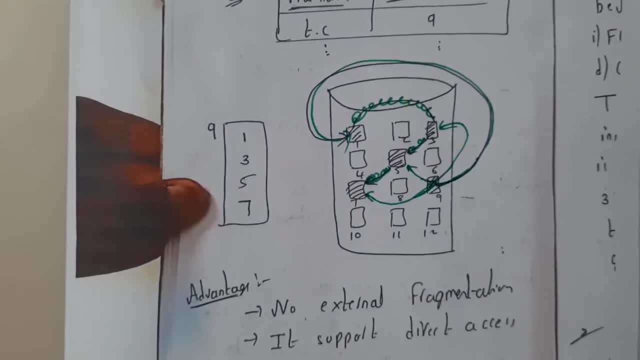 but once you are going through the definition, you'll be understanding it. sorry, once you are going through the example, you'll be understanding it. don't worry guys. okay, so this is a really easy way to do this. so let's go ahead and really easy and simple guys, simple way of allocation. so in the question he will. 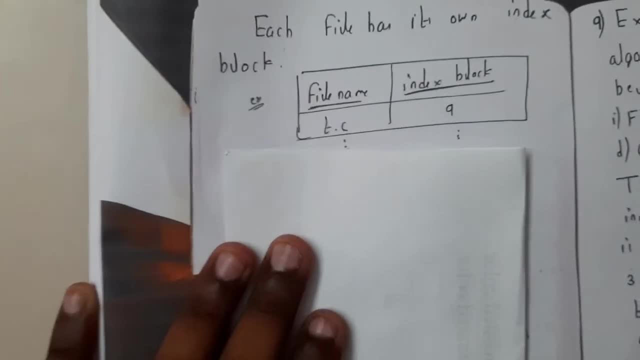 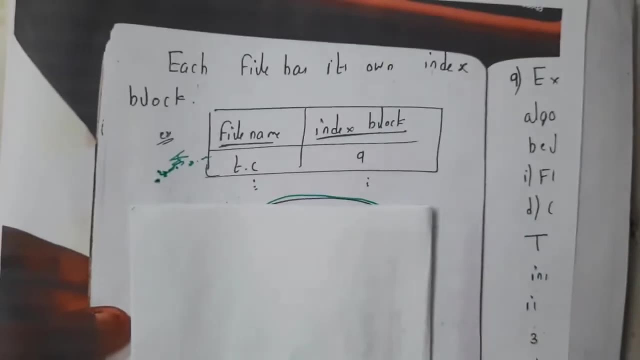 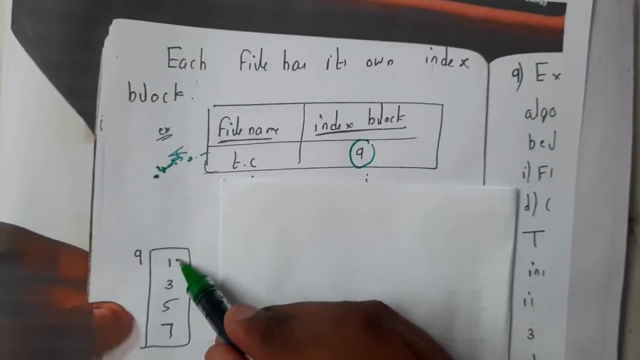 be giving that. the file name is just a second. just a second, guys. sorry for that, guys, okay. so basically the given question will be in this way: he'll be giving the file name and he will be giving the location of the block and the block will be having a particular links, so it is having from one, three, five, seven. 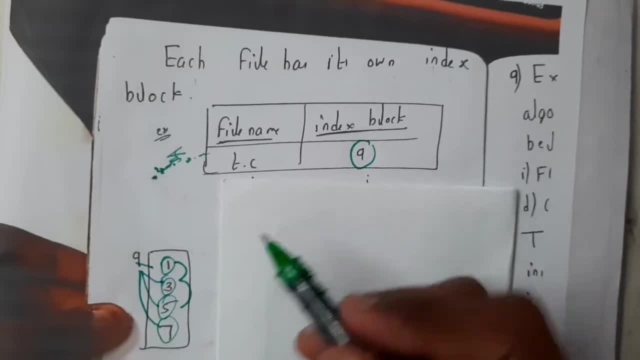 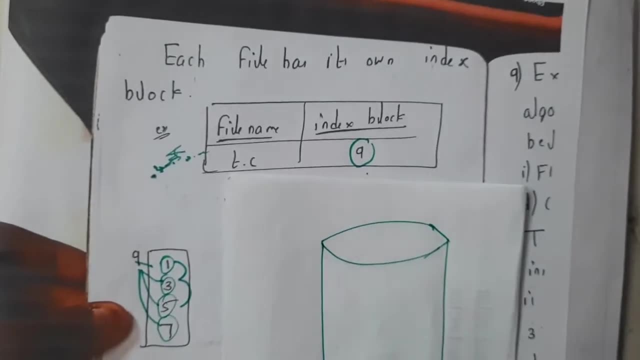 these are the links from the point nine. fine, okay, so for this we will be drawing in this way. so there are only eight, right, so we can just draw a 90. let me try. okay, zero one, two, three, four, five, six, seven, eight. I think that with all we need 9, also 9, 10, 11. fine, 1, 2, 3, 4, 5, 6, 7, 8, 9, 10.